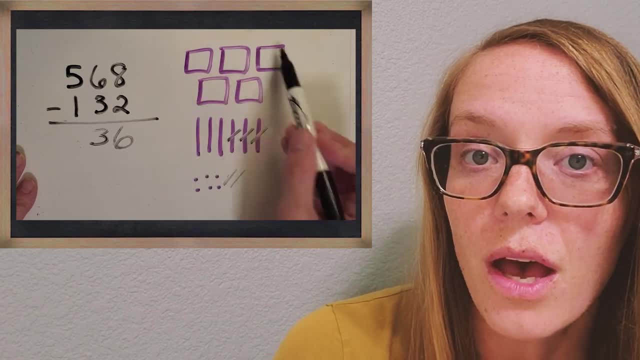 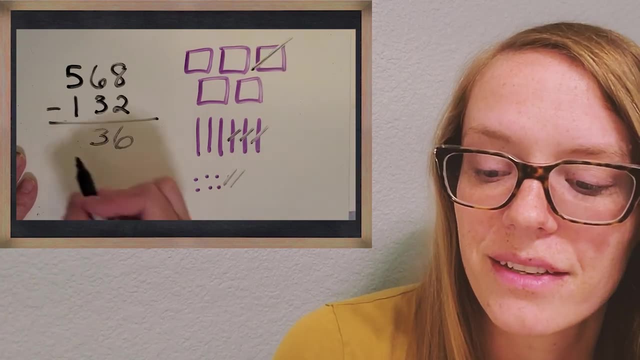 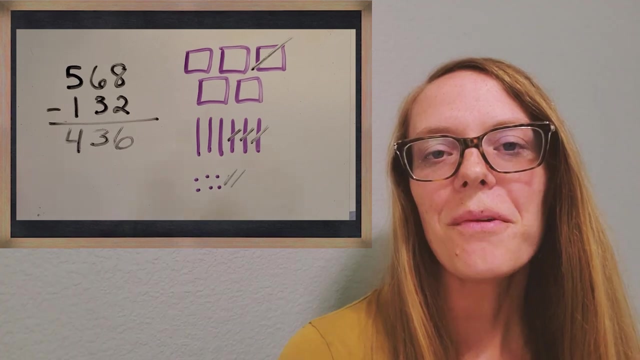 3 in that tens place, Then do the same thing with the hundreds place. So we have 5 flats and we just want to take away 1.. What do you have left? Okay, great, 4.. So we have 436 as our answer, Alright. 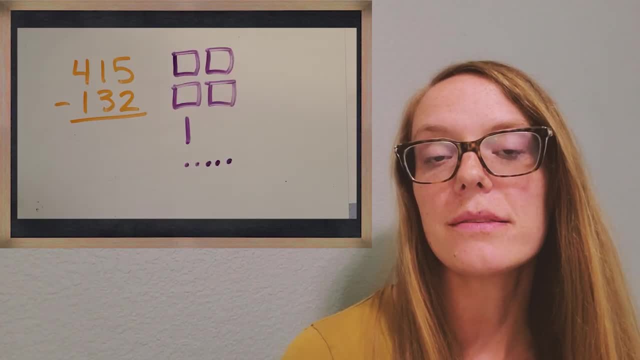 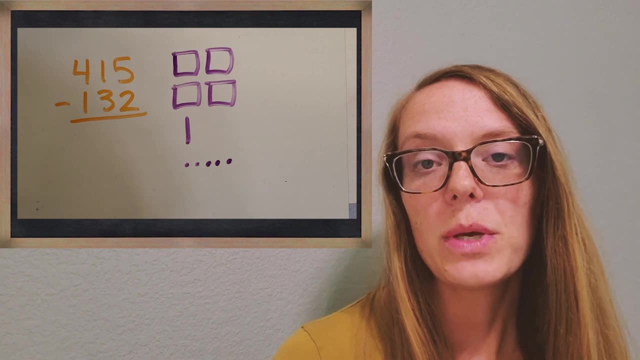 now I want to do a problem that has some regrouping in it, Since we're going to be working with subtractions. I know that's one of the biggest objectives with subtraction in third grade, So we need to try one where we need to regroup a little bit in order to do it. So I'll show you an example. 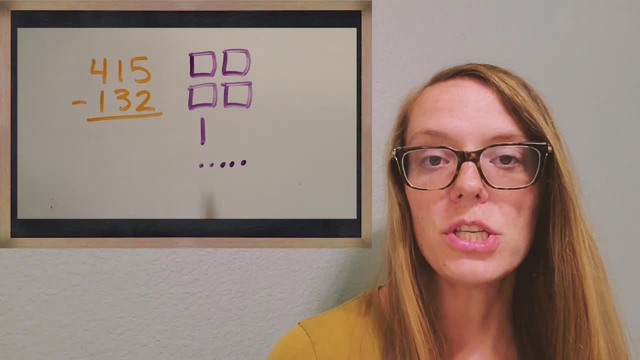 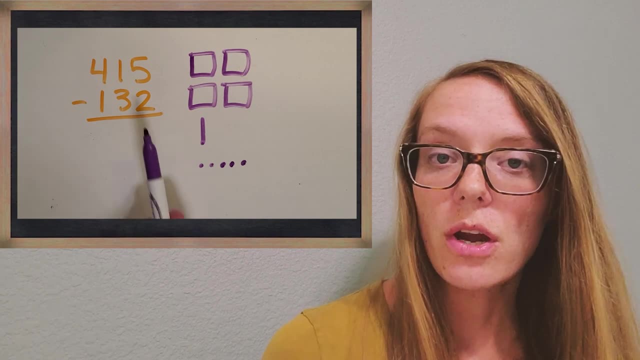 We have 415 minus 132, and the base 10 blocks can help us figure that out. So we're going to still start in the smallest place value. So what is 5 minus 2?? We can always take away 2.. 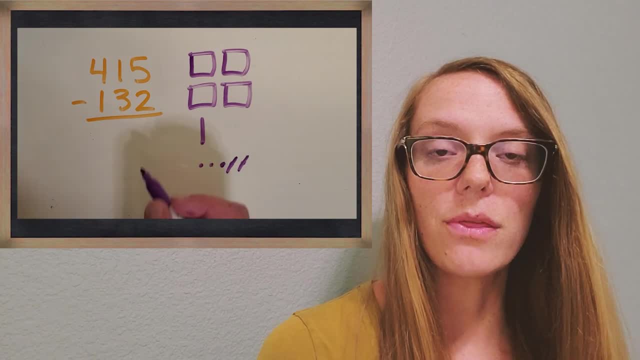 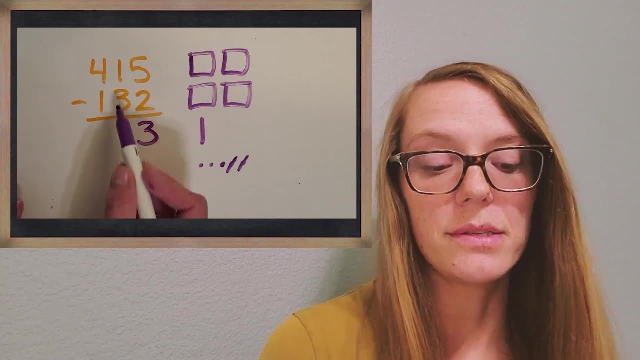 So we have 3 units. Okay, great, you got 3.. And so there's really no regrouping in that place. Let's move over and see what happens in the tens place. So we've got 1 long, but we want to take away 3. 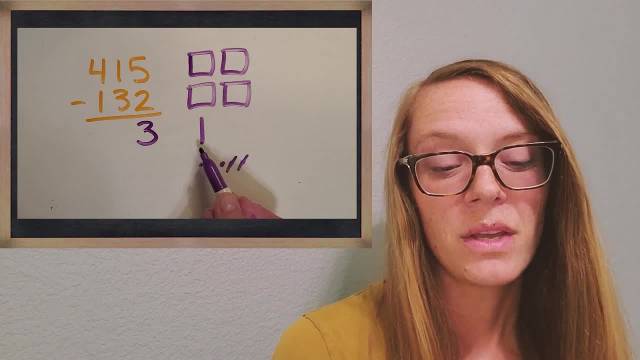 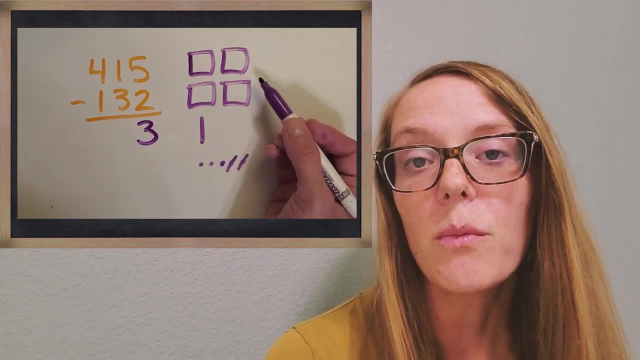 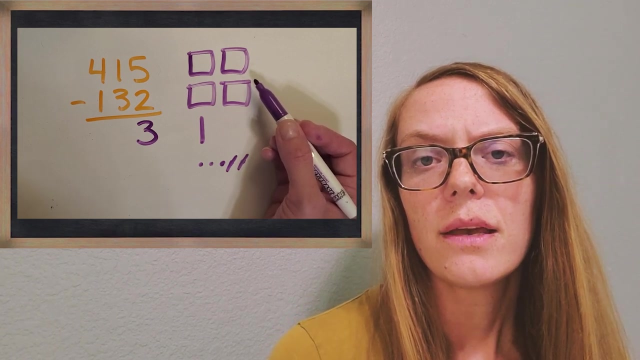 longs. That's where we're going to have a problem, huh. So we have a solution for that, though We can go over to the next biggest place value, and we can do what I like to call a trade or group. So let's look over at those flats. If I took one of them, what can I break it up into? 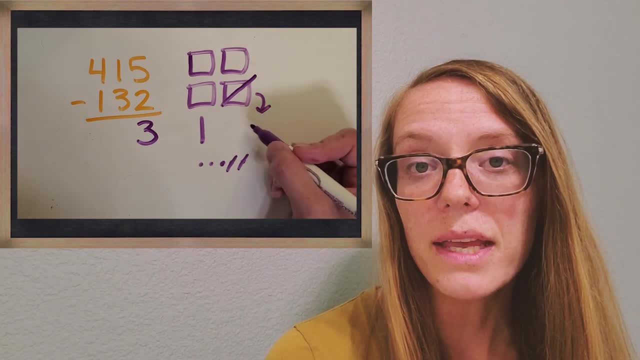 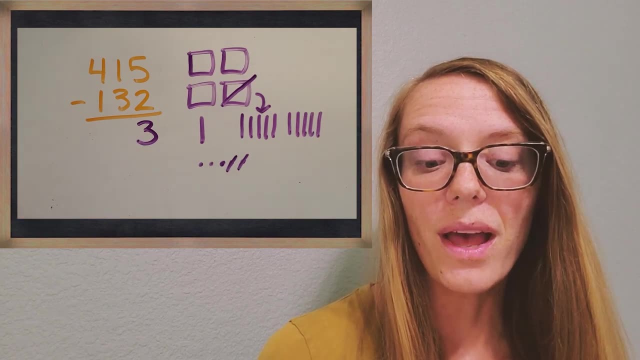 that might help. Yeah, I can break it up into 10 longs, So I'm going to make that trade really quick. Now I've got 11 longs, I can definitely take away 3.. So it just it helps me because 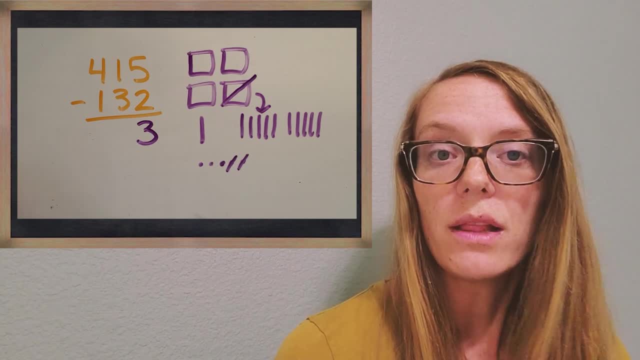 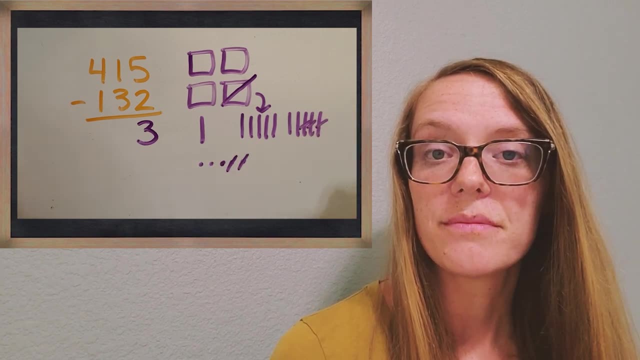 then I can subtract And I'll show you the way it looks in the algorithm too. right there, So now 11, let's take away 3.. How many do you have left? Okay, awesome, We have 8 left.